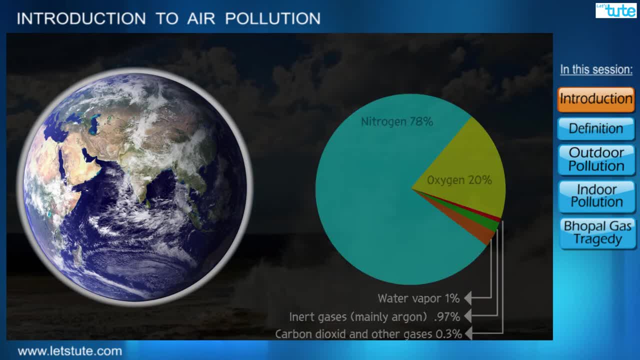 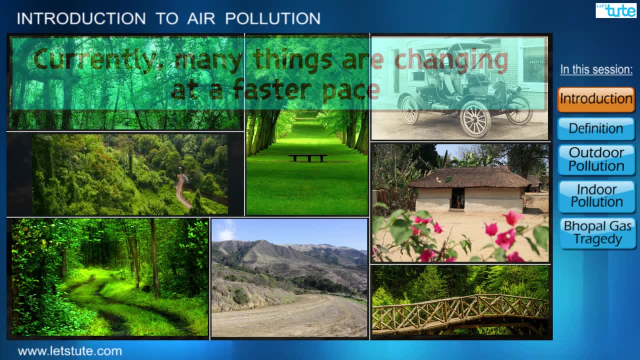 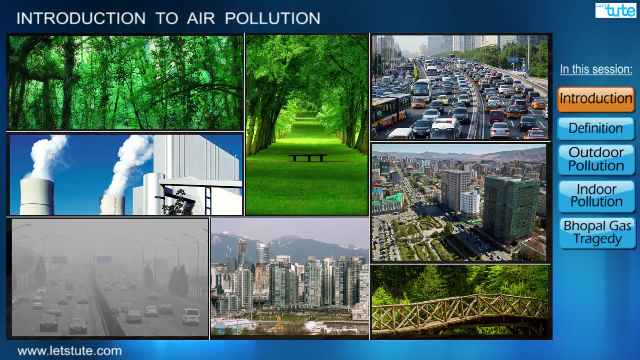 made up of many different components. currently, in this race for progress, many things are changing, and that, too, at a faster pace. industrialization, urbanization, more and more number of vehicles on street, changing lifestyle, have all led to deterioration in the quality of air, and we can say that the 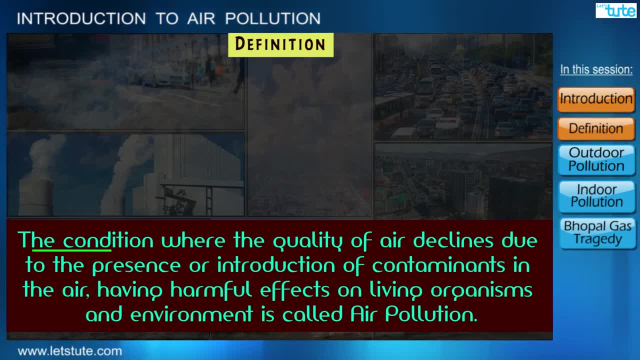 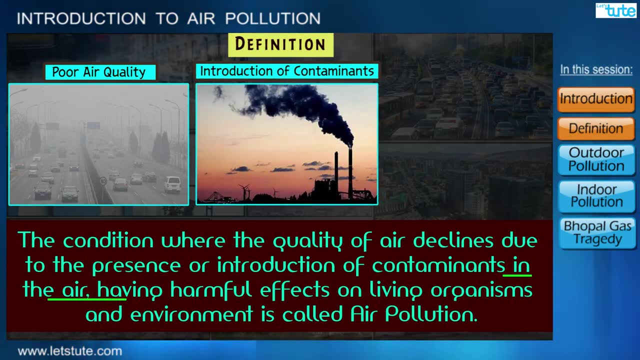 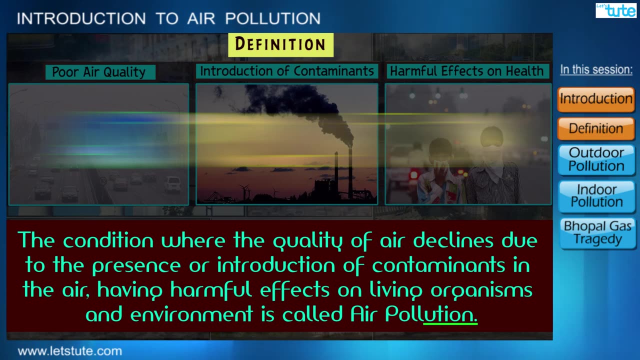 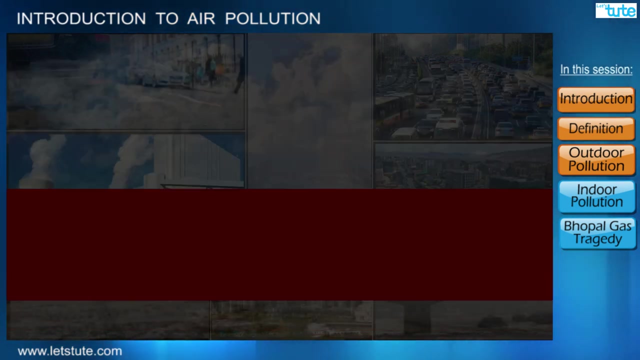 air is getting contaminated. so the condition where the quality of air declines due to the presence or introduction of contaminants in the air having harmful effects on living organisms and environment is called air pollution. friends, here our focus should be on the substances that are causing this pollution, or see the air pollutants. so tell me, where do these pollutants? 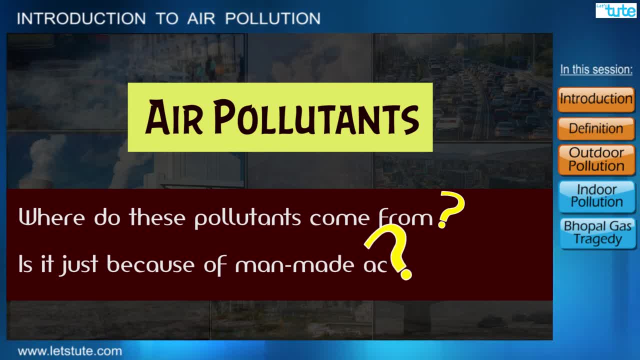 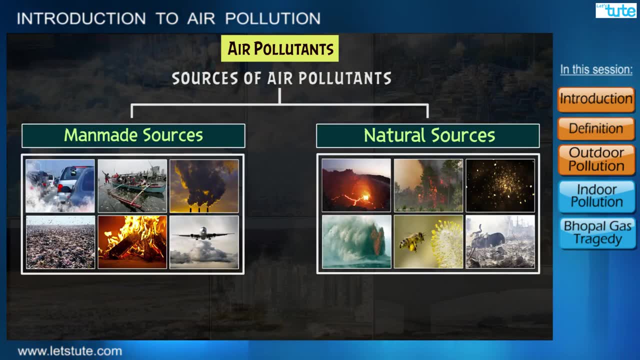 come from? is it just because of man-made activities? no, pollutants can be, from both natural and man-made sources. volcanic eruptions, pollen grains, dust particles, forest fires are all examples of natural sources of pollutants, whereas man-made sources include the smoke from industrial processes, vehicular emission. 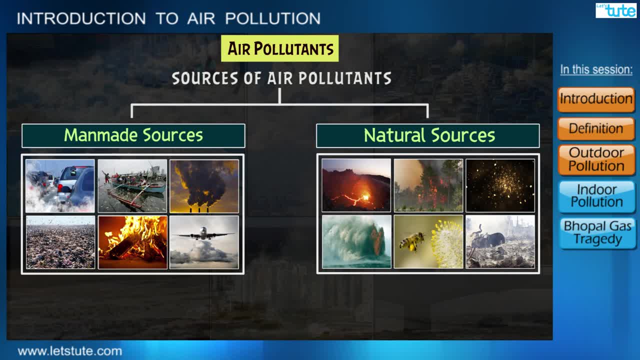 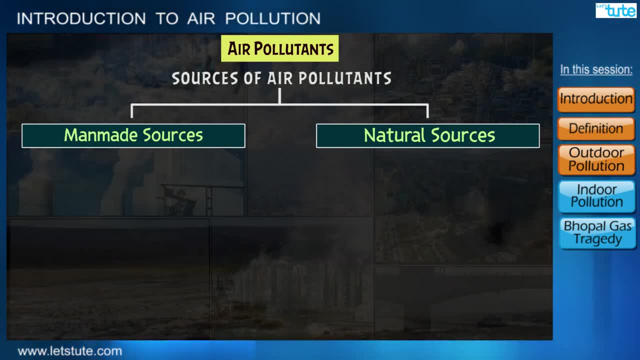 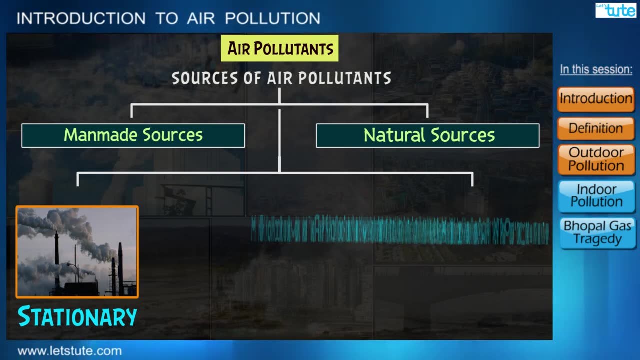 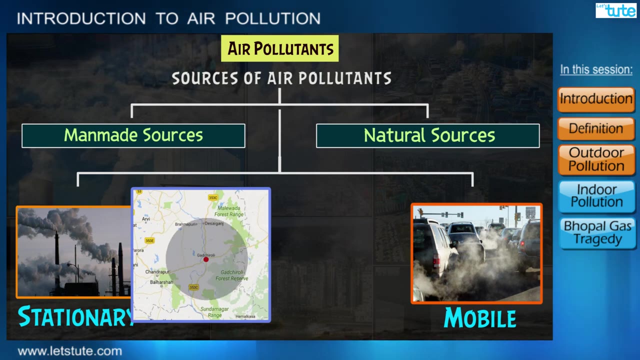 burning of firewood, etc. when we speak about the source of a pollutant, it can have a different perspective, like if the pollutant is coming from up point or stationery source, or is it coming from a non point or mobile source? now just consider the smoke coming from any factory. it will be an example of point. 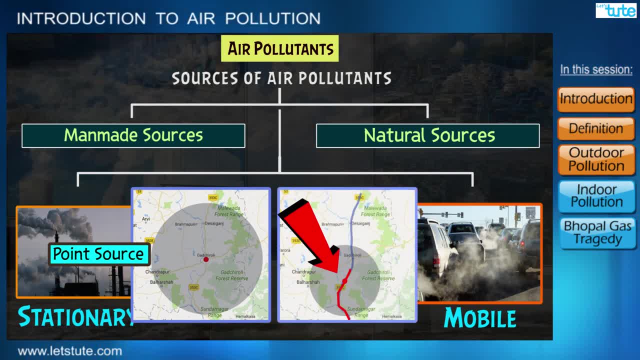 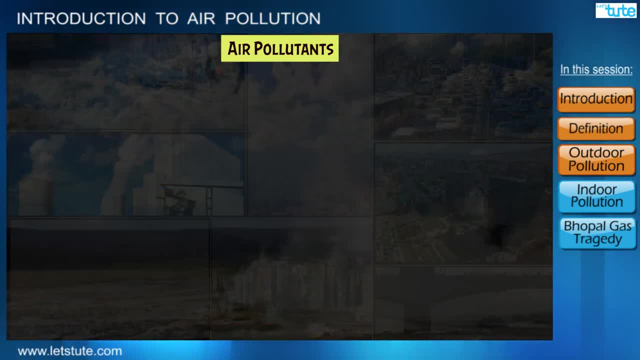 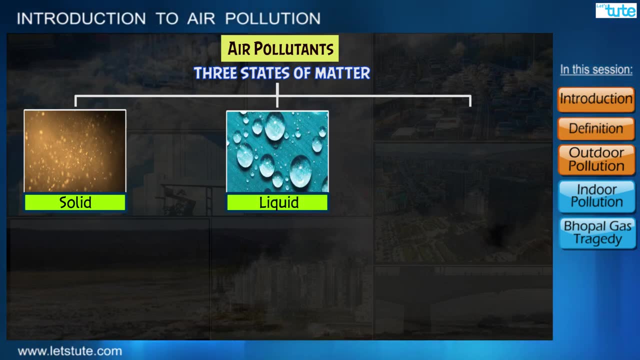 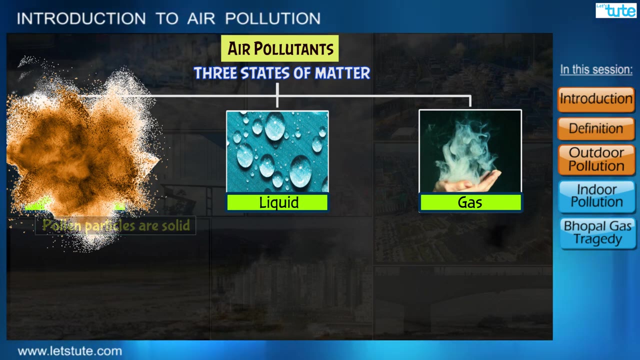 source, Whereas the fuel emissions of a moving vehicle will be a non-point source. And friends, these pollutants can exist in any three states of matter, ie solid, liquid or gas. See, for example, the dust or the pollen. particles are solid. 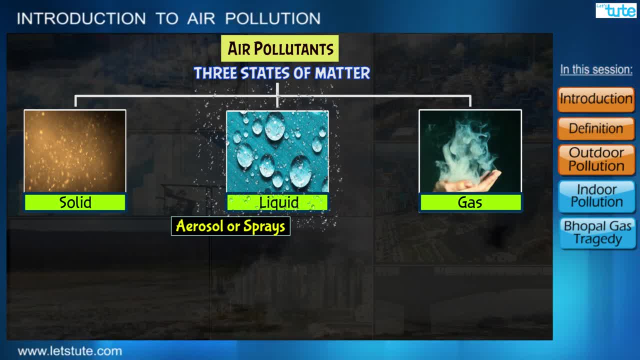 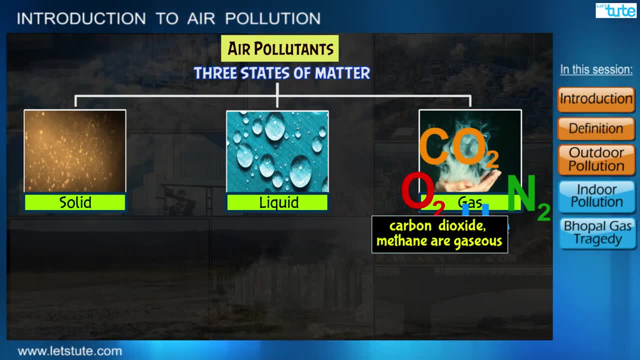 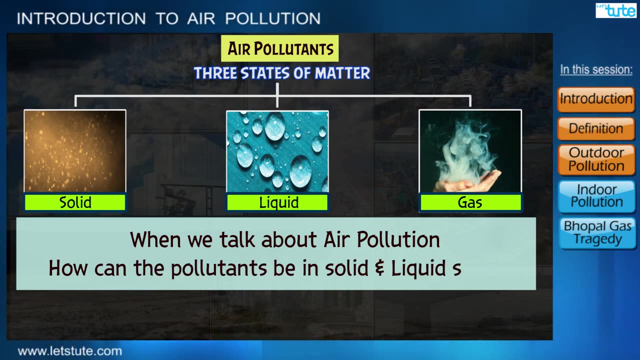 The aerosol or sprays that we use release tiny liquid droplets, And the various gases, like carbon dioxide, methane, are gaseous in nature. Generally, there is a misconception on how pollutants can be in all three states of matter when we are talking about air pollution. 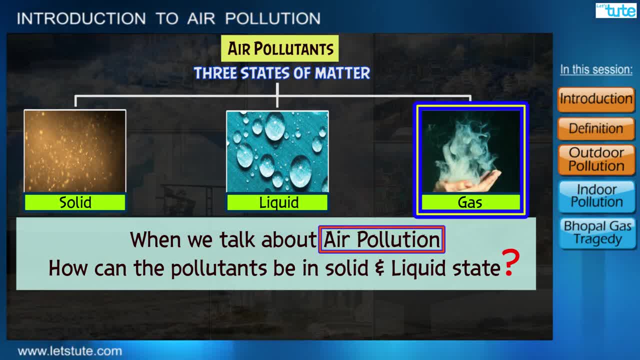 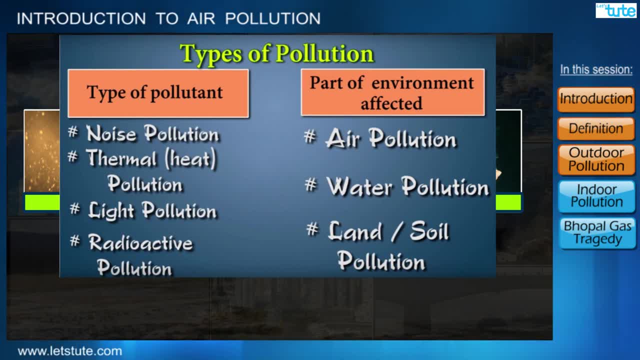 If it is air pollution, the pollutants should only be in gaseous state, right But no, Here the air habitat is not gaseous. Here the air habitat is not gaseous. The air habitat, ie the atmosphere, is getting polluted, and so it is called air pollution. 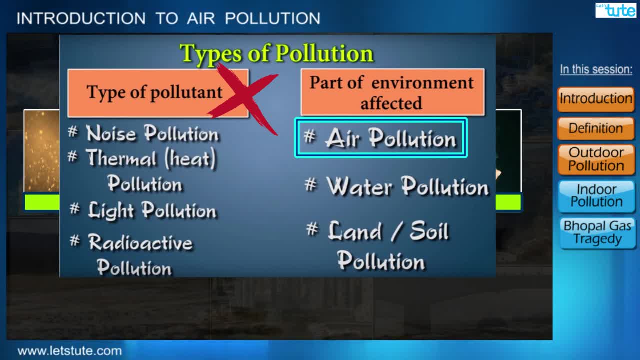 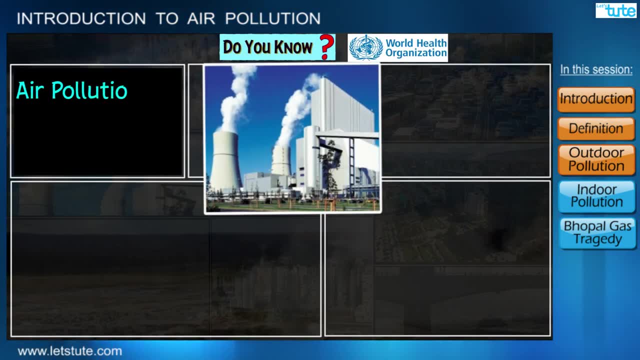 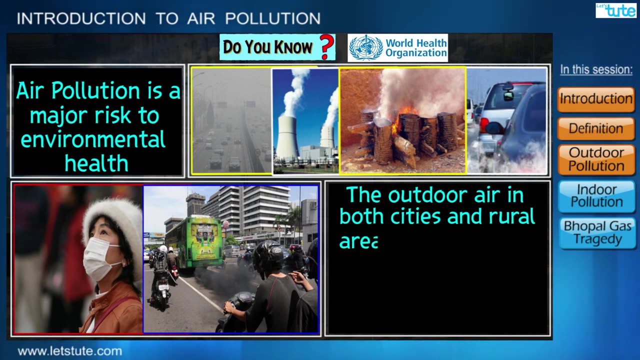 It is not on the type of pollutant that is introduced. I hope you are getting the difference. According to World Health Organisation, air pollution is a major risk to environmental health. The outdoor air in both cities and rural areas was estimated to cause 3 million premature. 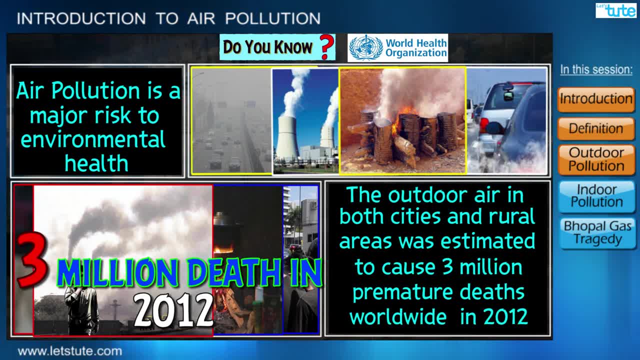 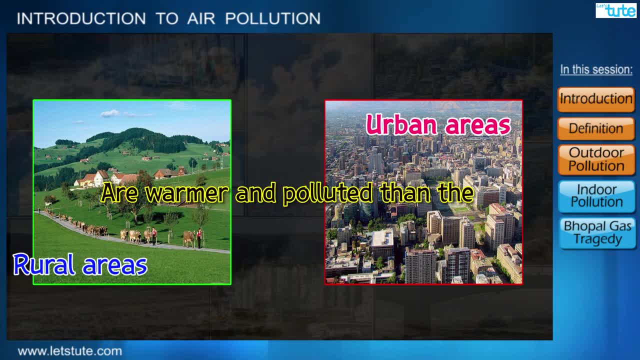 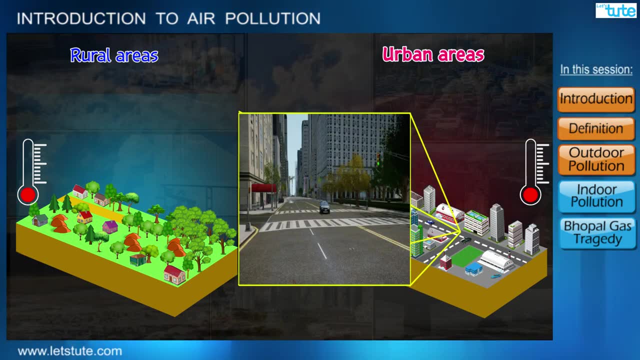 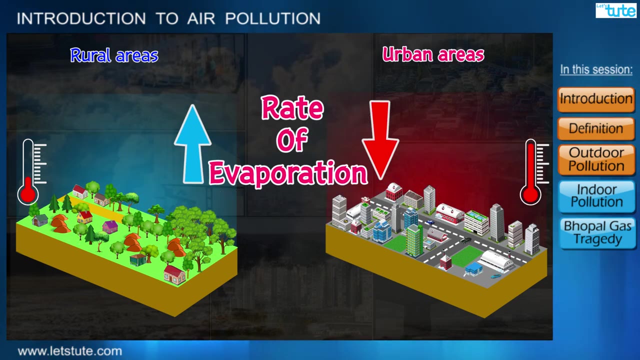 deaths worldwide in 2012.. But the crowded urban areas, especially the business districts, are warmer and polluted than the rural areas, Say. the infrastructure there, may it be the tall, dark buildings, roads, poor vegetation- absorb a lot of heat. The rate of evaporation, too, is low, and waste heat is emitted from vehicles, air conditioners. 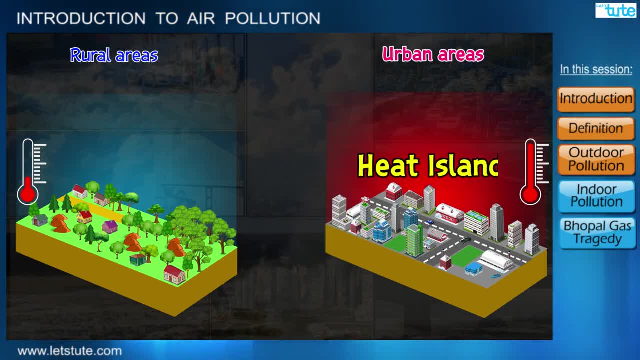 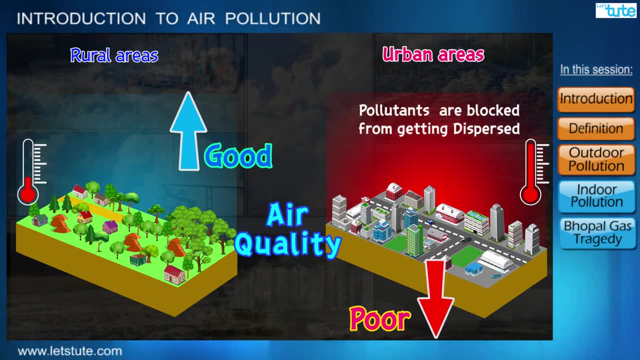 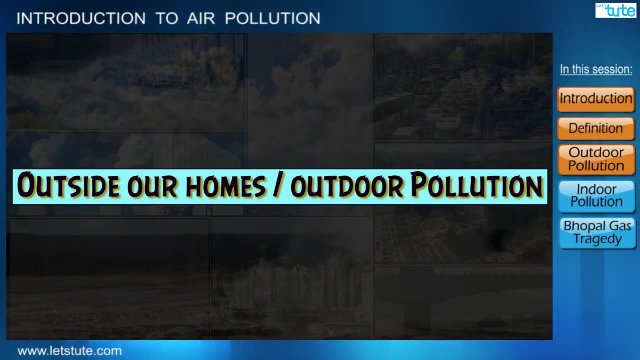 generators, thus resulting in the formation of heat islands. These areas have poor air quality as the pollutants are blocked from dispersing. All this while we spoke about the things that we see outside our homes. may it be the smoke, smog, vehicular pollutions, etc. 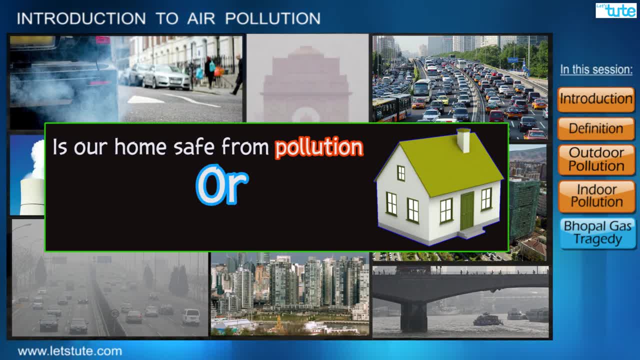 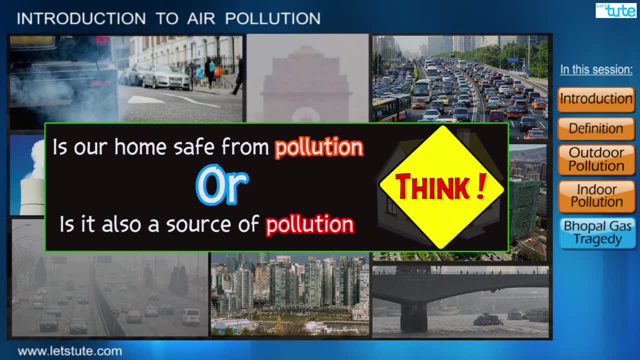 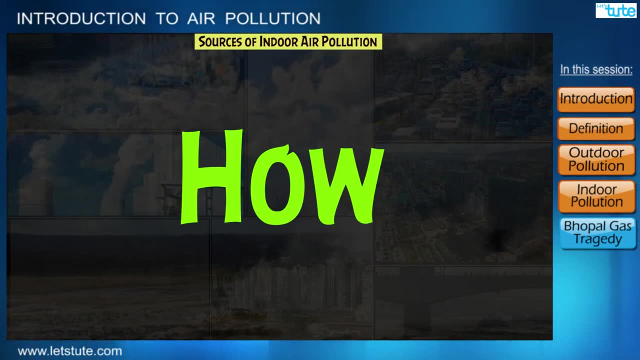 But is our home safe from pollution, Or is it also a source of pollution? This is something for us to think on, right. Whether we realize or not, air indoor can also be polluted, Wondering how? Let me give you some examples. 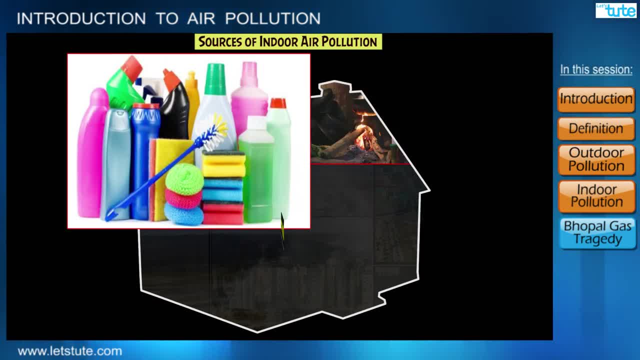 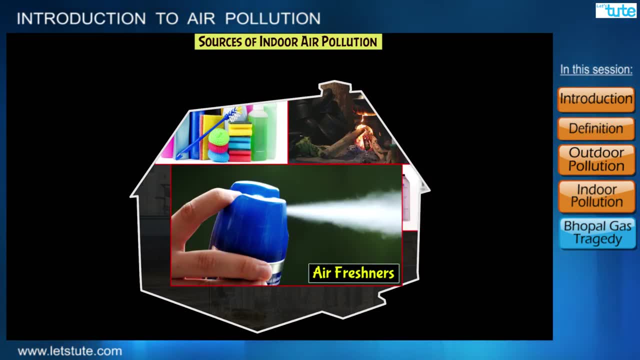 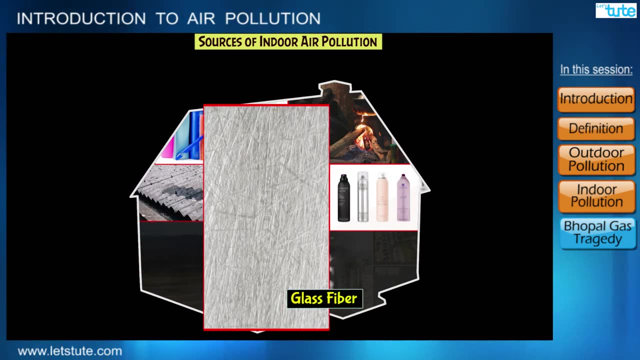 Cooking and heating of our homes. Use of urban household chemicals for cleaning, The use of various perfumes, hair sprays, air fresheners release a lot of chemical contaminants in the air. The building materials like asbestos, glass, fiber, paints and varnishes have health hazards. 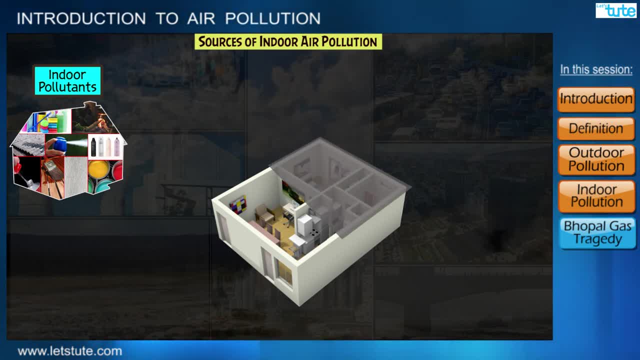 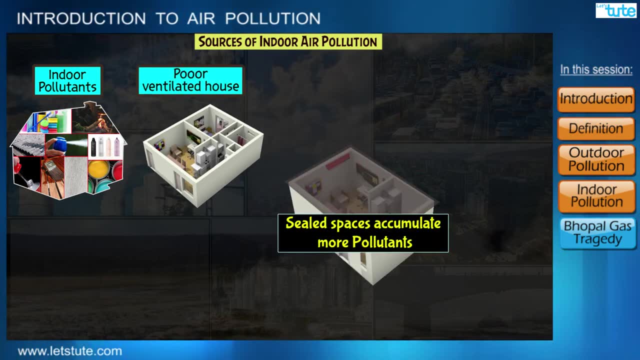 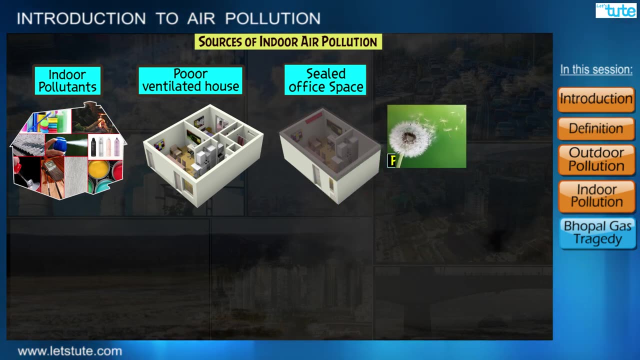 Moreover, the houses are small and many of them lack proper ventilation. The sealed spaces in offices and the air conditioned rooms accumulate more pollutants, again affecting the health Many a times: pollens from plants, mites from the hair of pets, fungi, parasites and some. 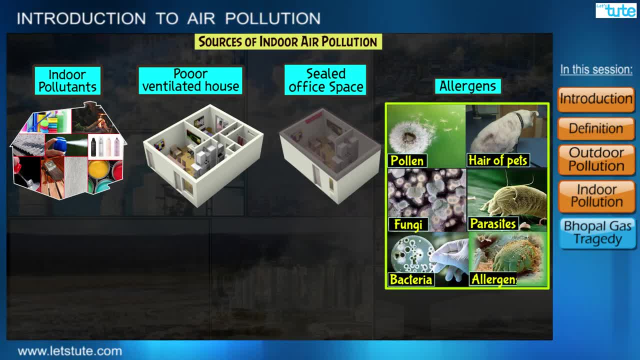 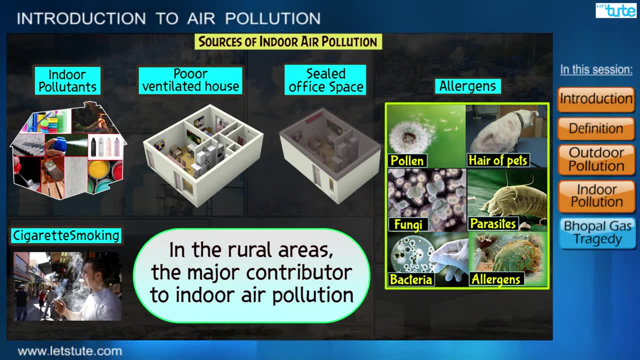 bacteria are polluted. For example, the smell of the air is present, which acts as allergens. Further, cigarette smoking can affect both smokers and non-smokers. In the rural areas, the major contributor to indoor air pollution is the use of fuel. 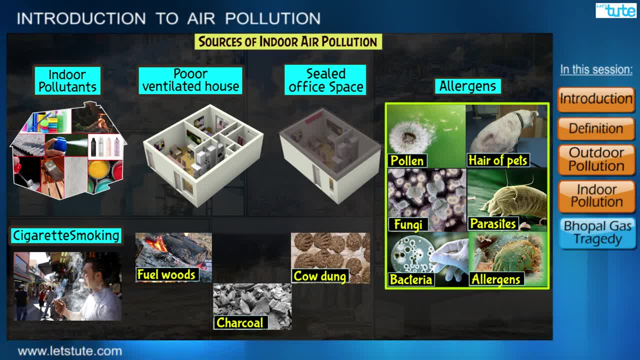 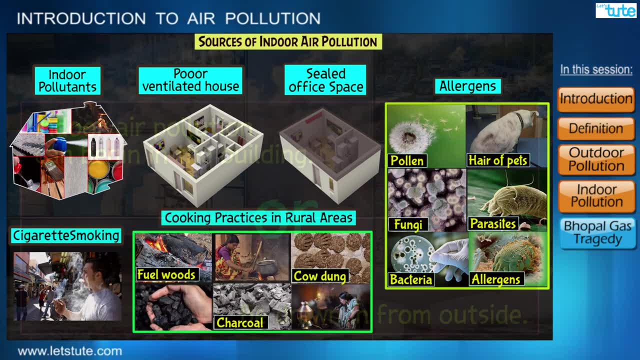 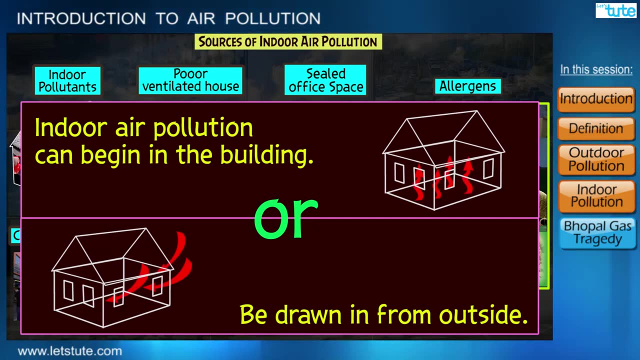 words: charcoal cow dung for cooking that produces a lot of smoke emitting large amounts of carbon particles. Indoor air pollution can begin in the building. It can also start in the building, But what is the use of indoor air pollution? or may be drawn in from outside. 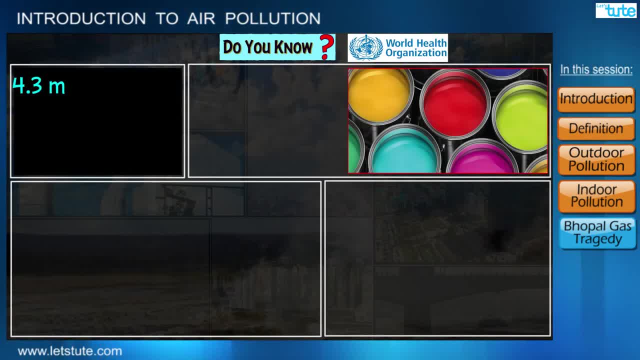 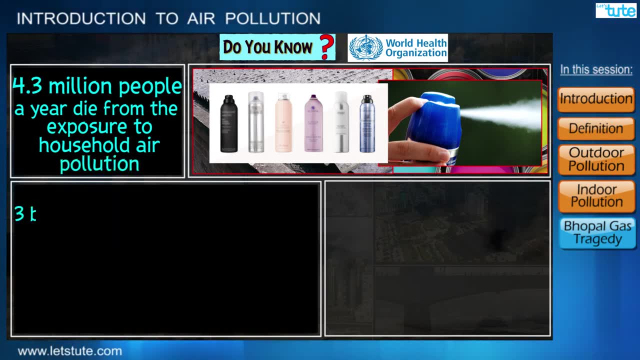 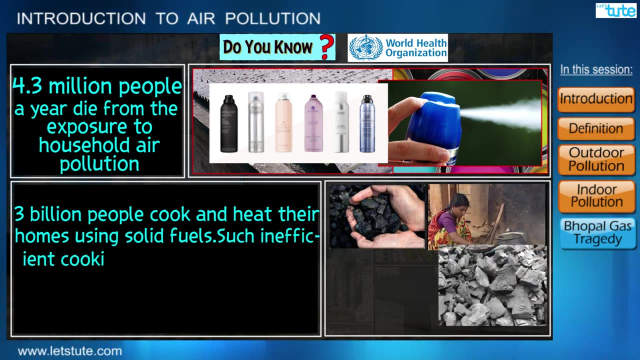 According to World Health Organization, 4.3 million people a year die from the exposure to household air pollution. Around 3 billion people cook and heat their homes using solid fuels. Such inefficient cooking and heating practices produces high levels of indoor air pollution. 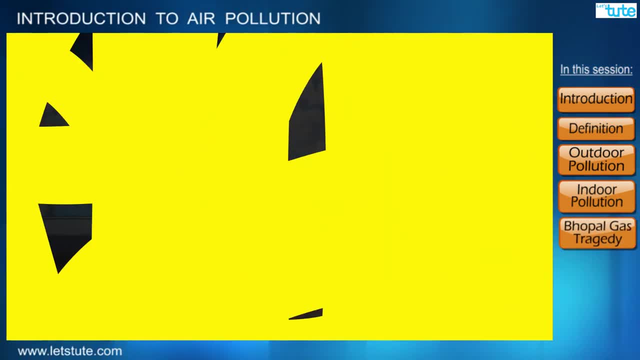 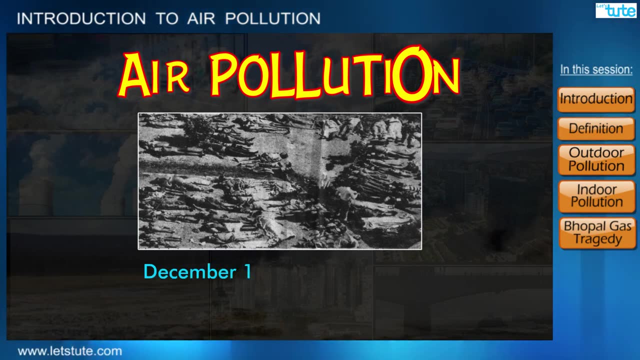 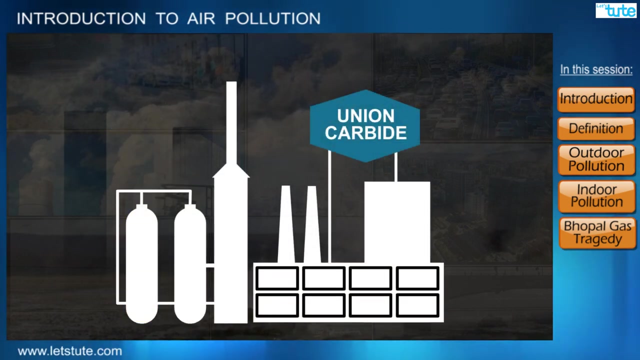 When we are talking about air pollution, we cannot miss to remember this catastrophe which took long back in the year 1984 in Bhopal, India, which is also known as the Bhopal gas tragedy: 40 tons of toxic gas was accidentally released from Union Carbide plant.